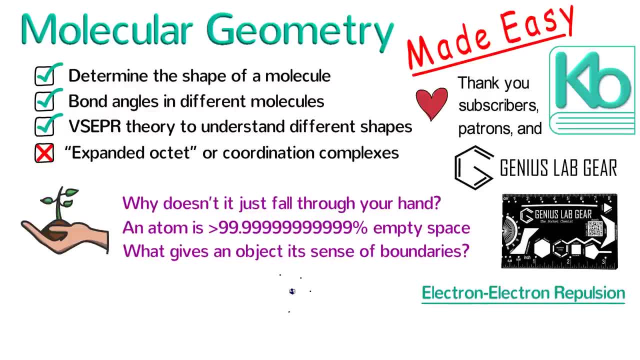 Its sense of boundaries. Electron-electron repulsion: When an atom approaches another atom, the negatively charged electrons of the two atoms repel each other. So the size and boundaries of an atom are determined by electrons repelling each other. That same principle also determines the shape of a molecule. 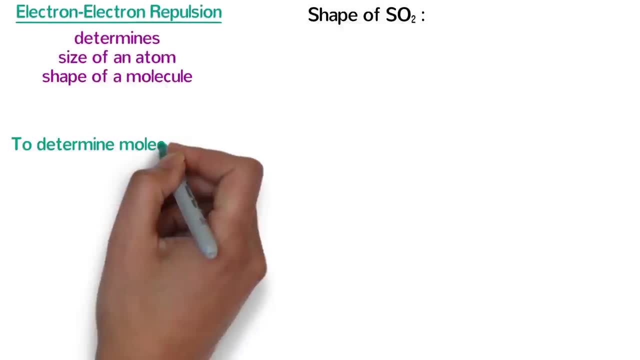 Let's see how this works in the example of sulfur dioxide. The first step in determining the shape of a molecule is to draw the Lewis diagram, And if you don't know the Lewis diagram already, you'll have to count the valence electrons. 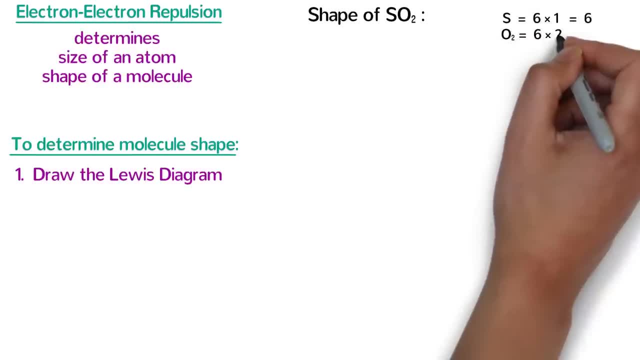 One sulfur has six valence electrons and the two oxygens have six times two or twelve valence electrons, which gives sulfur dioxide a total of eighteen valence electrons. Because there is only one sulfur, we put sulfur in the middle, surrounded by two oxygens with single bonds to the sulfur. Each bond has two electrons. 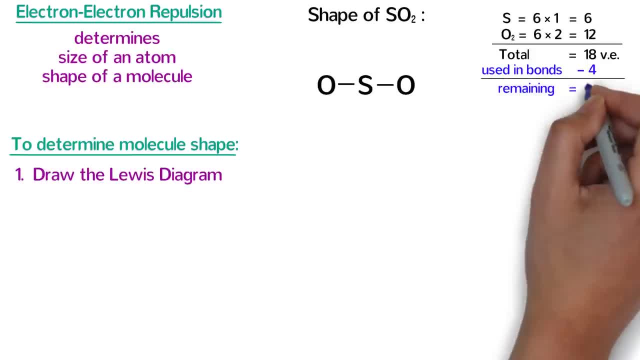 so we have used up four electrons so far, which means we have fourteen electrons remaining for lone pairs: Two, four, six, eight, ten, twelve and fourteen. Notice that the sulfur has only six valence electrons around it, so we should use two of 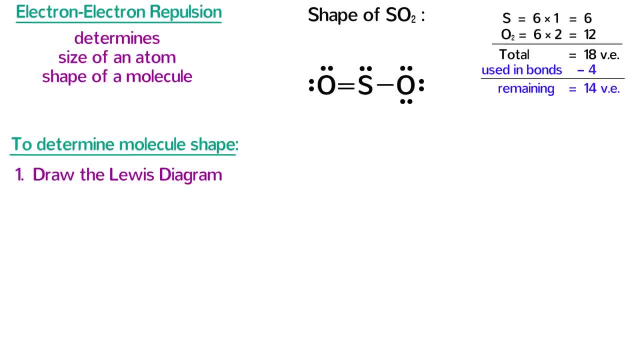 oxygen's electrons to form a bond between it and sulfur. The resulting Lewis diagram is complete, with each atom having eight valence electrons. After you draw the Lewis diagram, you need to count the number of things on the central atom. By things I mean bonded atoms or lone pairs. 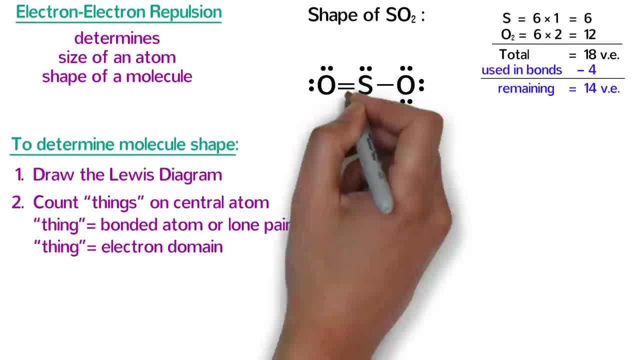 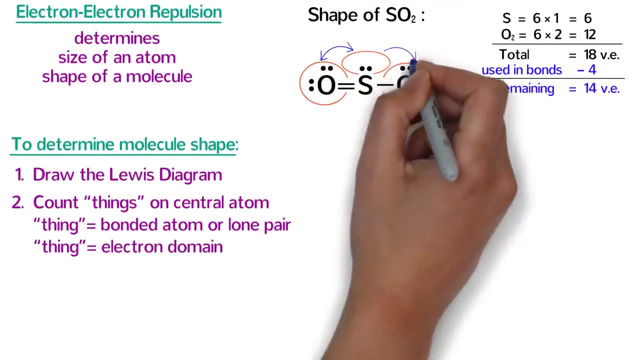 Technically speaking, these are called electron domains. The double bonded oxygen is a thing, as is the single bonded oxygen and the lone pair on the sulfur. Remember that only lone pairs on the central atom count. so there are three electron domains, or things on sulfur dioxide that determine its shape. 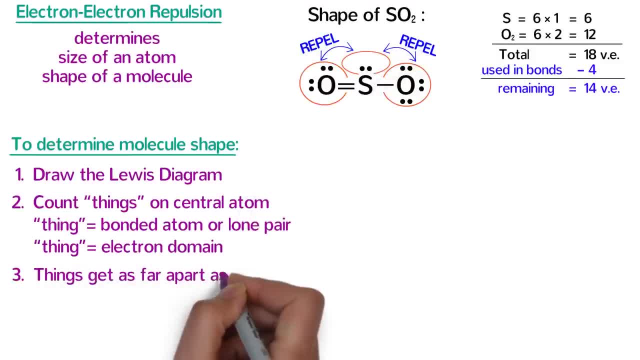 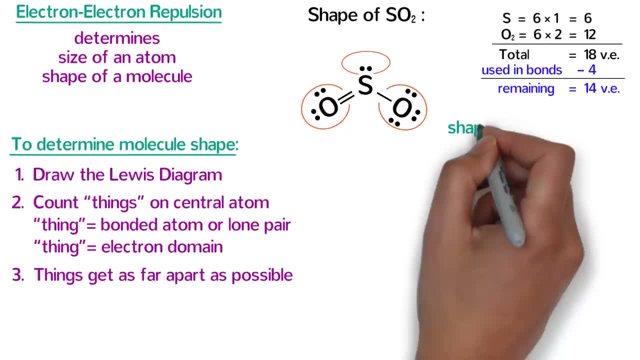 Those three things will repel each other and get as far apart as possible. That repulsion with a lone pair of electrons will cause the two oxygens to bend down, so the resulting shape of SO2 is called bent, Since there are three things attached to the central atom. 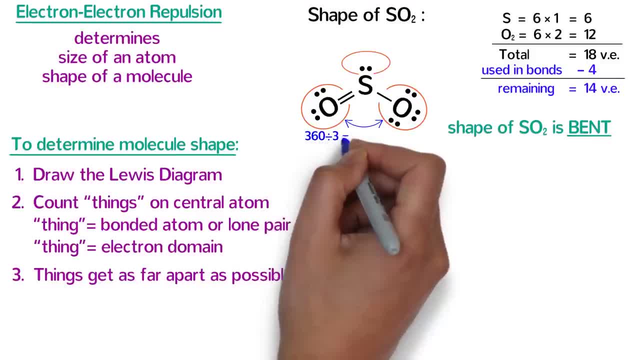 we would expect the bond angle to be 360 divided by three or 120 degrees. In fact, the real bond angle is slightly less than that. It is 19 degrees, because lone pairs occupy more space close to the central atom, while electrons and bonds are stretched out between the two bonding atoms. 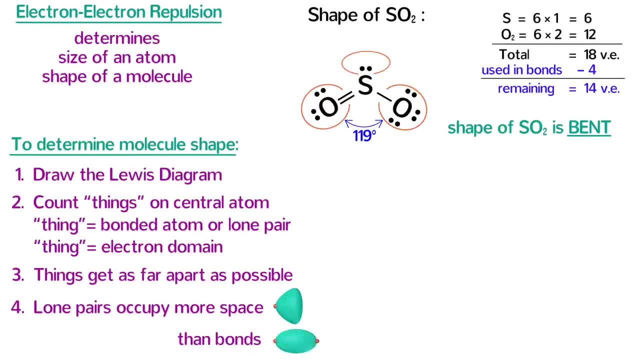 Okay, now let's try to apply these principles to determine the shape of several other molecules. Let's start with carbon dioxide. You may wish to pause the video now and try to draw the Lewis diagram and determine the shape of carbon dioxide on your own. 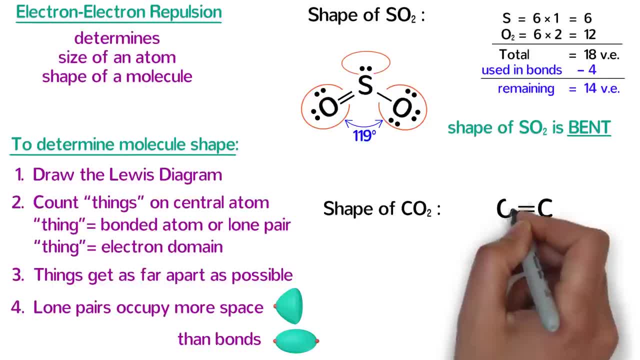 For the Lewis diagram. carbon is in the middle and it forms double bonds to each oxygen, which both make up the lone pairs. Next we need to count the number of things on the central atom. In this case there are only two things on carbon, Although there are lone pairs in the molecule. 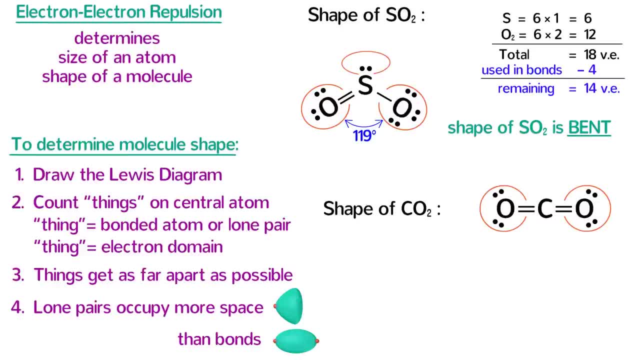 the lone pairs on oxygen do not affect the shape because they are not on the central atom. Since there are only two things, you can see in our drawing that those two things are already as far apart as possible Because the three atoms are all in a line. 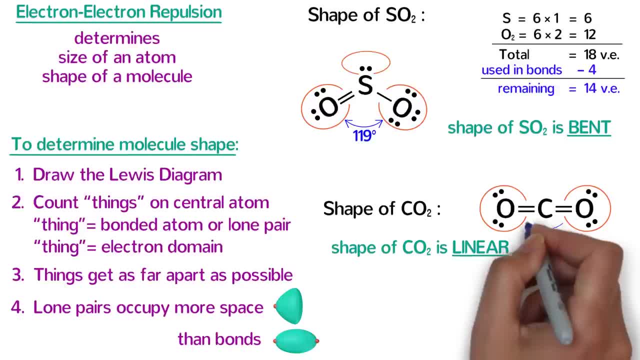 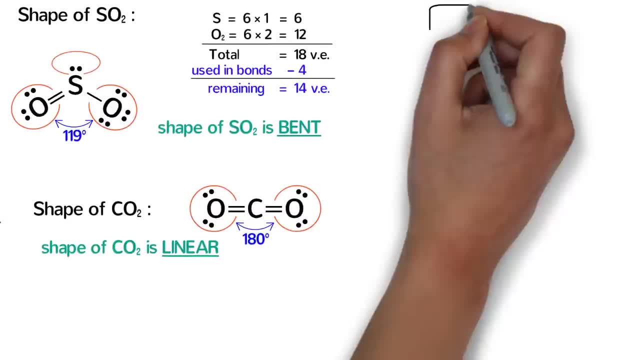 we say that the shape of CO2 is linear and the bond angle is a linear 180 degrees. As we take a step back and look at SO2 and CO2, we can see that for a three-atom molecule, the only two possible shapes. 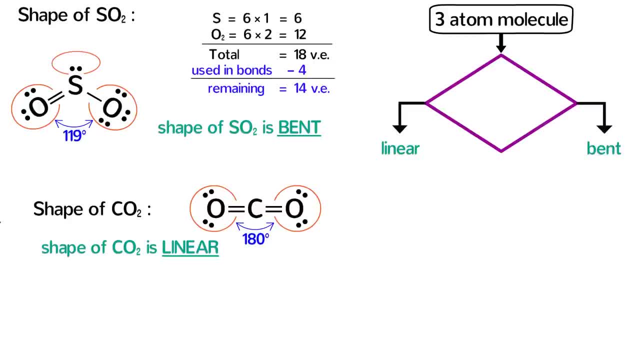 are linear or bent, and the deciding factor is whether or not there is a lone pair on the central atom. Bent molecules have one or more lone pairs in the central atom, while linear molecules have no lone pairs on the central atom. Before we move on to more complex molecules, 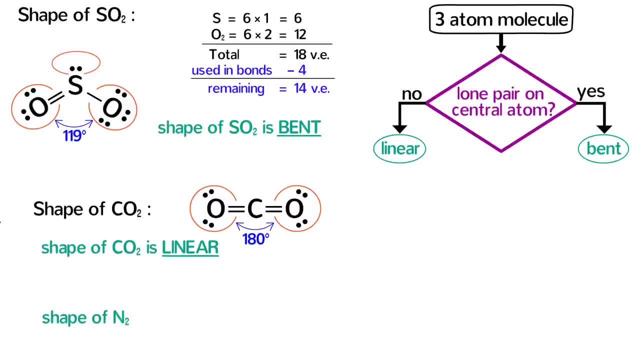 let's consider two-atom molecules such as N2.. Two-atom molecules do not have a central atom, which means they cannot have any bond angles. So the only possible shape for two atoms is linear. N2 is linear and all two-atom molecules are linear. 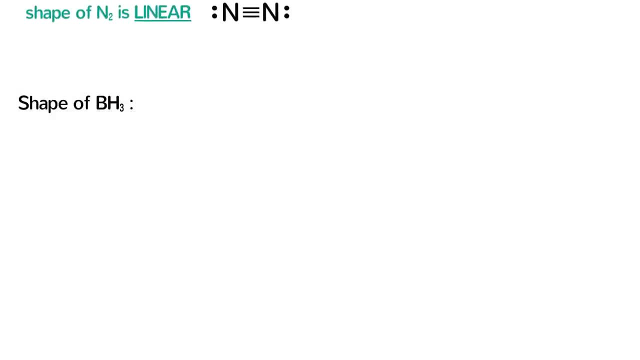 Next, let's look at some four-atom molecules like boron trihydride. When drawing the Lewis diagram of BH3, boron is in the middle and it makes three single bonds to the three hydrogen atoms. Remember that, because boron starts with only three. 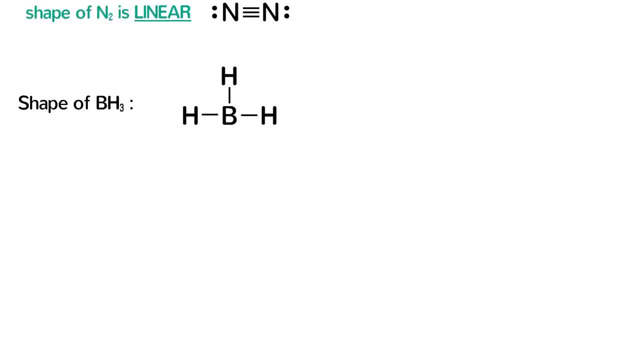 valence electrons and each hydrogen starts with one valence electron. there are no more electrons in the central atom, So boron is in the middle and it makes three single bonds to the three hydrogen atoms. Boron has three things around it and each of those things will repel each other to get as 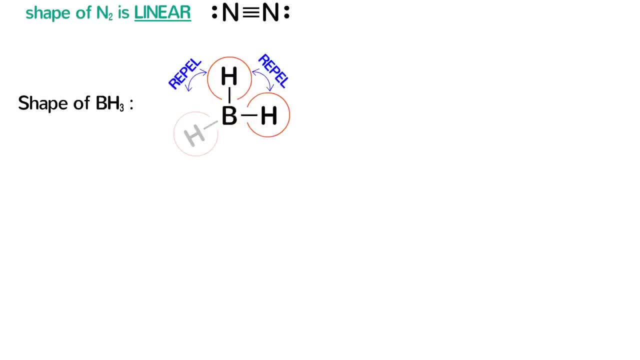 far away from each other as possible. That repulsion will lead to a symmetrical structure with all the bond angles being equal. That is all. the bond angles are 120 degrees and the molecule is perfectly flat without any puckering. Because the molecule looks like a flat triangle? the name: 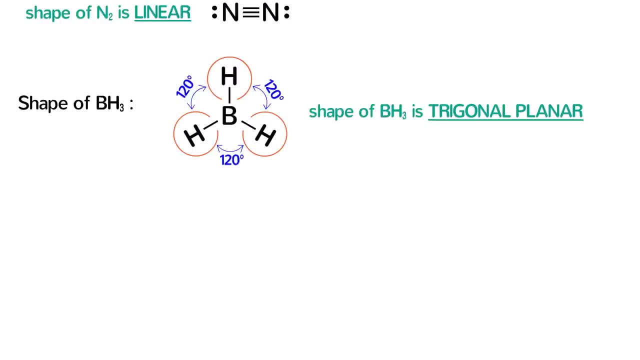 of its shape is trigonal planar. Let's try another four-atom molecule, CH2O. That is for maldehyde. Because carbon prefers to make four bonds. we put carbon in the center, Each hydrogen only forms one bond and oxygen prefers to form two bonds. That leaves four electrons for lone pairs. 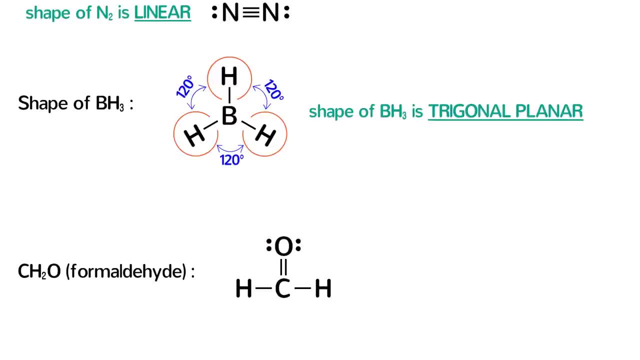 which both go on the oxygen to give every atom an octet or a duet. There are three things on the central atom and those three things repel each other. Once again, we can see that the molecule looks like a flat triangle, so the shape is trigonal, planar. However, the bond angles are 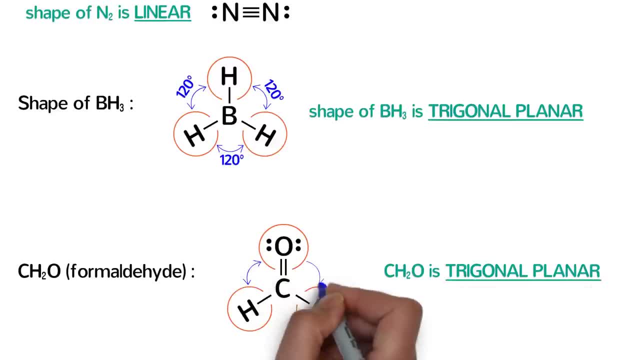 not exactly 120 degrees. The HCO bond angles are pretty much the same. The HCO bond angles are both 122 degrees. They are a little bit bigger than 120 because double bonds occupy more space than single bonds. The HCH bond is consequently only 116 degrees. Remember that a double bond has 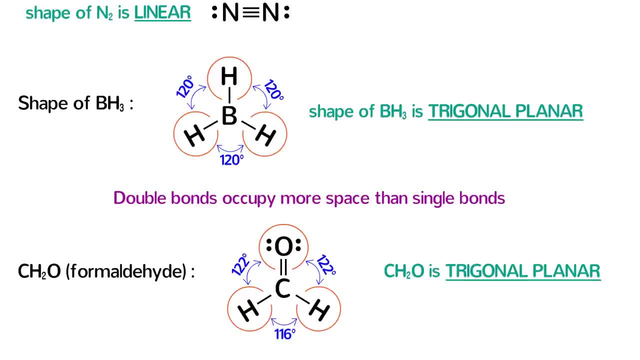 four electrons, and a single bond has two electrons, so the double bond would repel more and need more space than a single bond, but the shape is still the same. Next, let's check out a five-atom molecule like CH4. That is methane. Carbon is in the middle, with four single bonds to 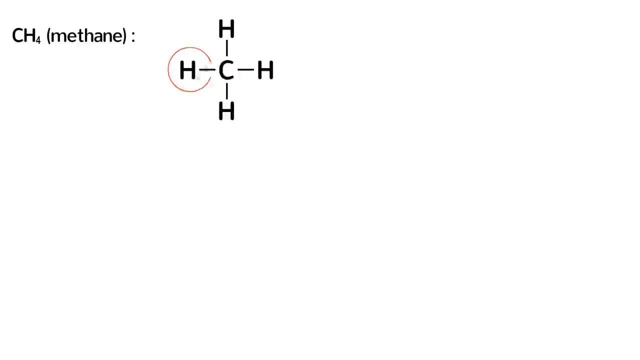 hydrogens, and there are no lone pairs. Now there are four things on the central atom, and each of those things will repel each other to be as far apart as possible. This time it appears as though they are already as far apart as possible, and it appears as though the bond angles should all be. 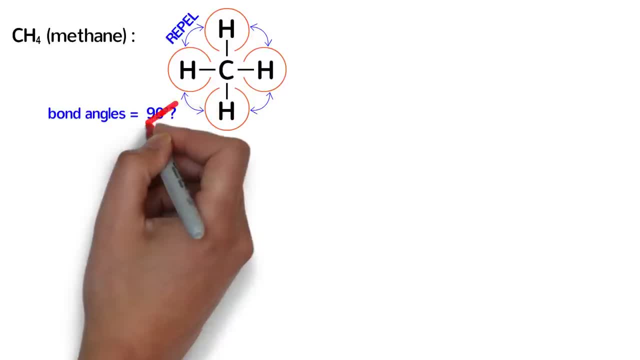 90 degrees. However, looks can be deceiving when you are trying to visualize a three-dimensional molecule on a two-dimensional surface. The hydrogens can actually move away from you or towards you in three-dimensional space. The resulting shape is not flat. 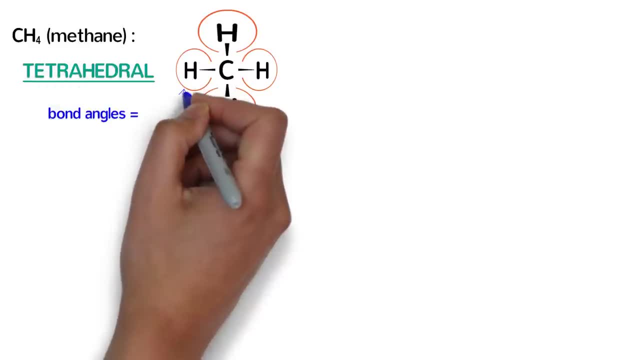 a three-dimensional shape called tetrahedral, and the bond angles are consequently larger than 90 degrees. The bond angles are all 109.5 degrees. It can be difficult to visualize this shape, so I recommend that you build methane in similar molecules yourself with a physical 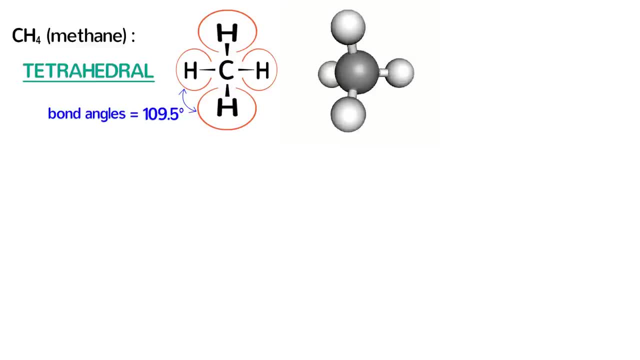 molecular model or an application like MoleView. Here is a ball and stick 3D model of methane. Notice the bond angles and the symmetry of the molecule. To give it a bit of a three-dimensional perspective, methane is sometimes drawn like this or like this: The dashed bond. 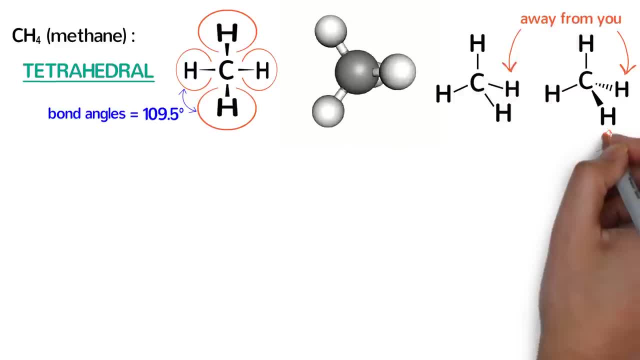 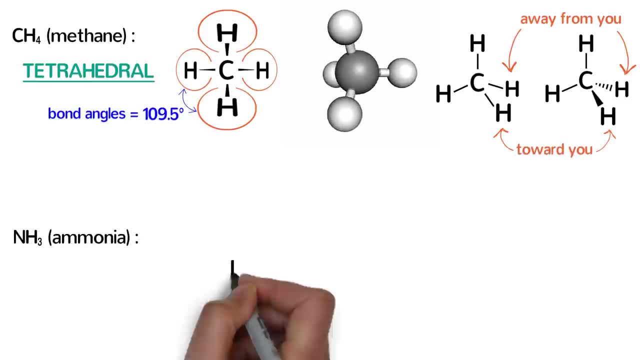 represents a bond that is going away from you, while a solid wedge bond represents a bond that is going toward you. Next, let's try NH3, which is called ammonia. Unlike BH3, which we said was trigonal planar, NH3 has a lone pair of electrons on the central atom. In some ways, ammonia is. 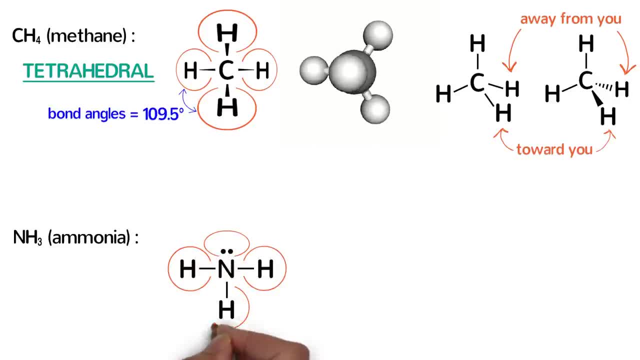 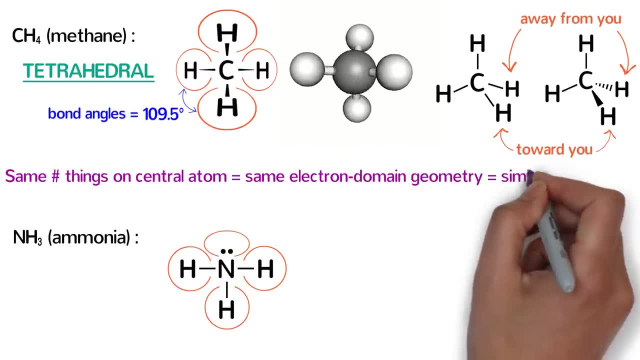 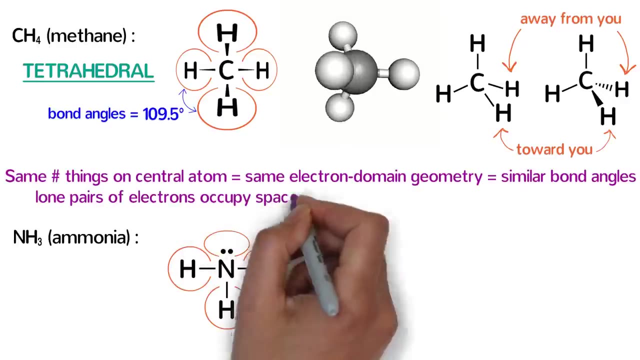 similar to methane because it also has four things attached to a central atom. In general, molecules that have the same number of things on the central atom are said to have the same electron domain, geometry and tend to have similar bond angles. However, actual shape of these molecules will differ because lone pairs of electrons occupy space. 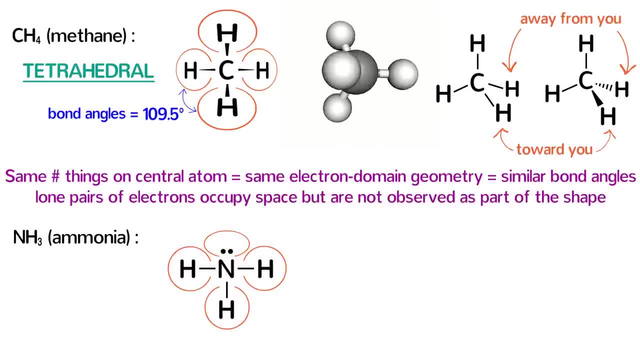 but are not observed as part of the shape. As for ammonia, those four things attached to nitrogen will all repel each other and because there are four things attached to the central atom, just like in methane, we expect that the bond angles will be about 109.5.. We can represent. 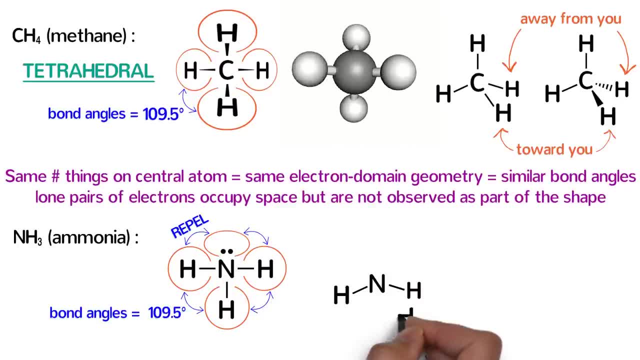 this three-dimensional shape the same way we did methane, only this time we put the lone pair on top. Here is a ball and stick model of ammonia. Its shape is called trigonal pyramidal because it essentially looks like a pyramid with a triangular base. You can think of trigonal. 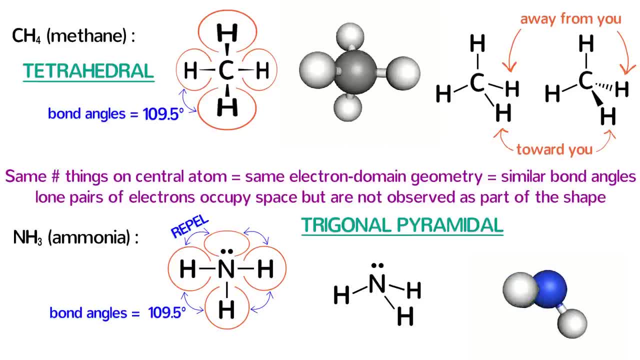 pyramidal as tetrahedral with one atom removed. or you could think of trigonal pyramidal as trigonal planar with the central atom pulled up. some For ammonia, the actual bond angle is very close to 109.5, but it is a little bit smaller because lone pairs occupy more space close to the 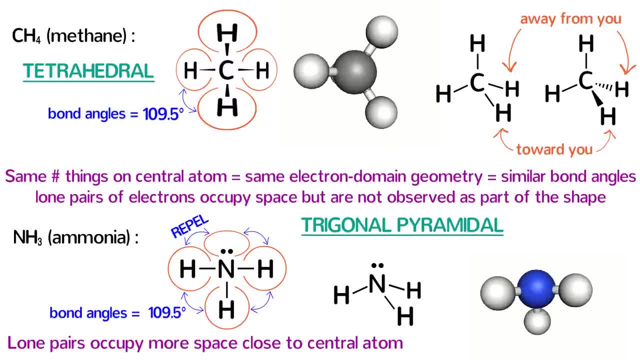 central atom, causing the hydrogen atoms to squeeze closer together. The actual bond angle of ammonia is 106.7 degrees. Okay, let's move on to the next one. Ammonia's bond angle is 106.7 degrees. We have already looked at the five basic shapes of molecules, along with an example for each one. 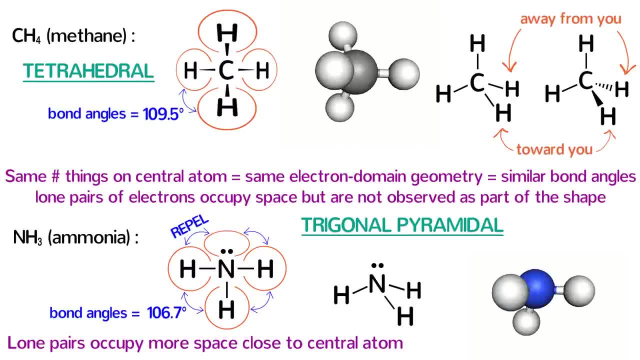 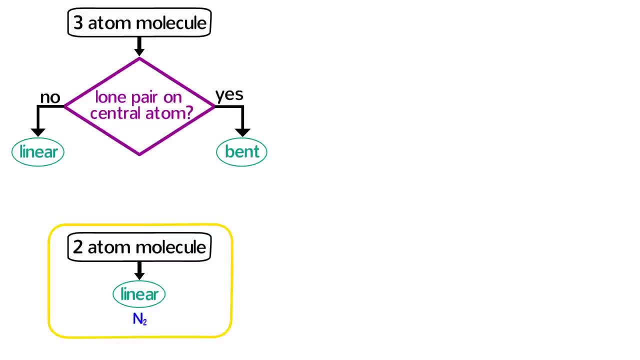 and the guiding principle of electron-electron repulsion. Let's take some time to summarize all this before we go through one last example: molecule. Previously we said that two atom molecules like N2 are always linear. If a molecule has three atoms, there are two possible shapes. 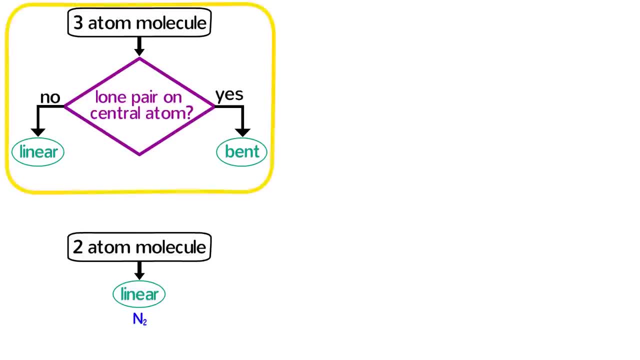 If there are no lone pairs of electrons on the central atom, the shape is linear, like CO2.. But if there are lone pairs the shape is bent, like SO2.. For four-atom molecules the shape also depends on whether or not there is a lone pair of electrons on the central atom. 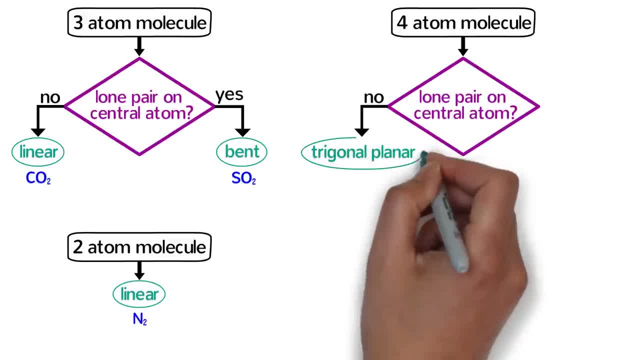 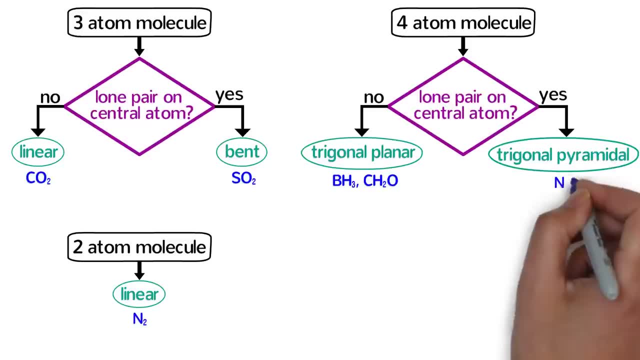 If there is no lone pair on the central atom, then the molecule is trigonal planar, like BH3 and formaldehyde. If there is a lone pair on the central atom, then the molecule is trigonal pyramidal, like ammonia. 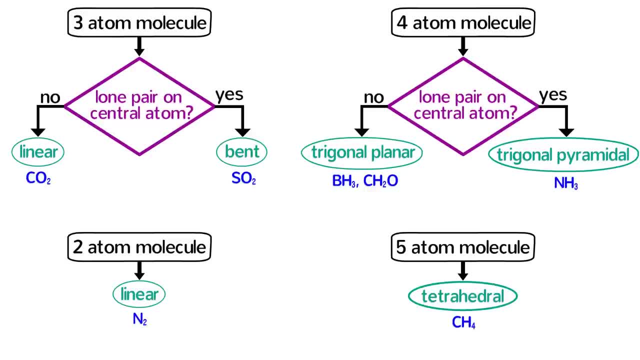 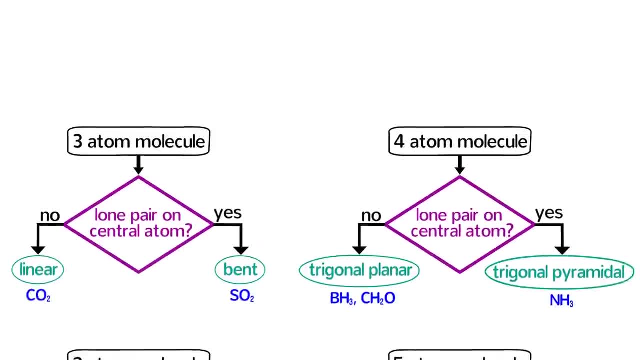 Lastly, five-atom molecules are typically tetrahedral, like methane, Although there are some exceptions. those exceptions are non-octet molecules, which I will discuss in a different video. Another way to summarize these shapes is by counting the number of things. 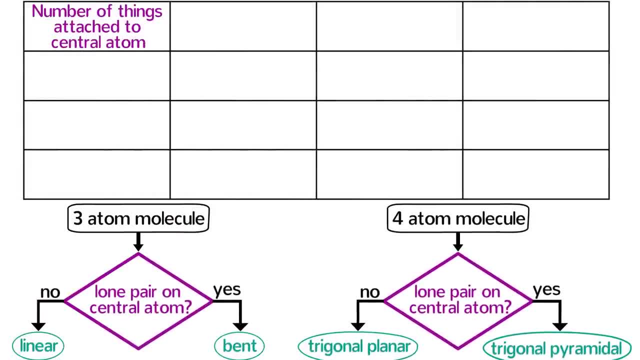 attached to the central atom. For example, in a three-atom molecule there are two atoms attached to the central atom. If there are zero lone pairs of electrons, the shape is linear and the bond angle is 180 degrees. If there is one lone pair, the shape is bent and the bond 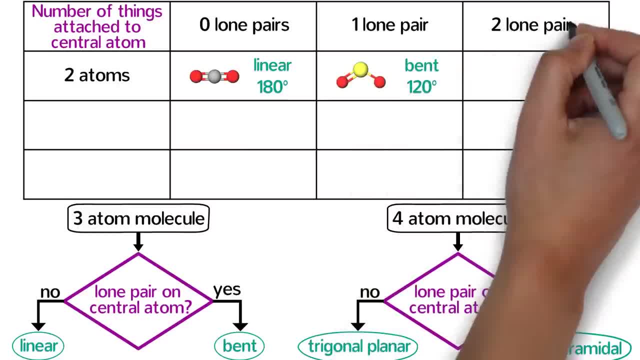 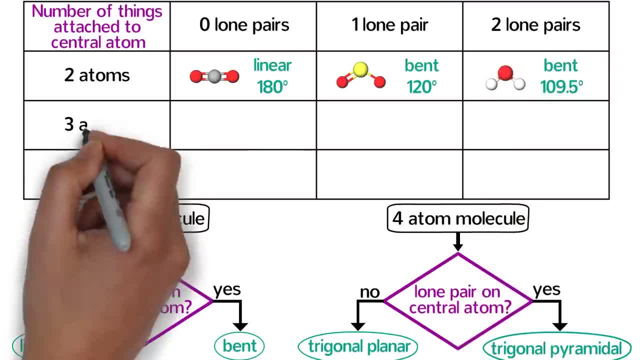 angle is approximately 120 degrees. If there are two lone pairs, the shape is also bent, but the bond angle is closer to 109.5 degrees. In a four-atom molecule there are three atoms attached to the central atom. If there are zero lone pairs on the central atom, the shape is trigonal. 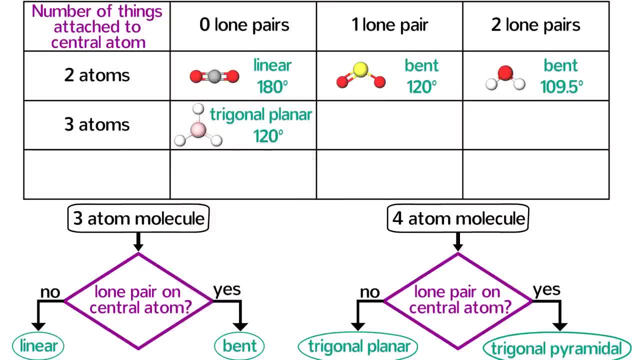 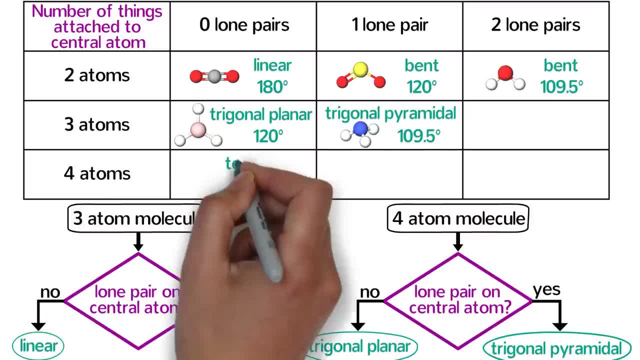 and the bond angle is about 120 degrees. If there is one lone pair, then the shape is trigonal, pyramidal, and the bond angle is about 109.5 degrees. Finally, if there are four atoms, the shape is tetrahedral and the bond angle is also 109.5 degrees. 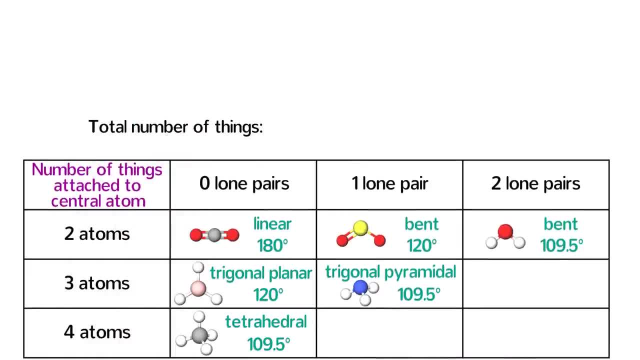 Notice that if the total number of things attached to the central atom is the same, then the bond angle will also be the same. A total of two things leads to a 180-degree bond angle, a total of three things leads to a 120-degree bond angle, and a total of four things on the central. 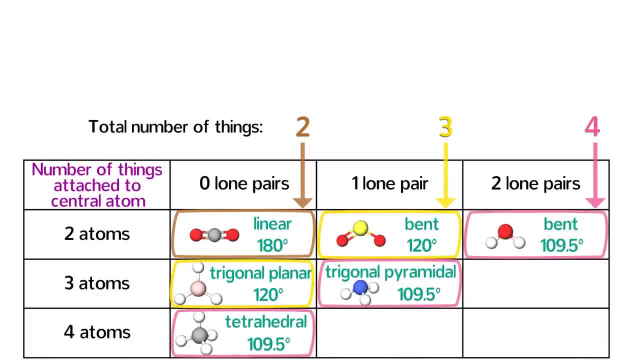 atom leads to a 109.5-degree bond angle. Now it's time for you to try a sample problem: What is the shape of H2O and what is the approximate bond angle? Pause the video and try to figure it out yourself. The first thing that you should have done is draw the Lewis diagram. 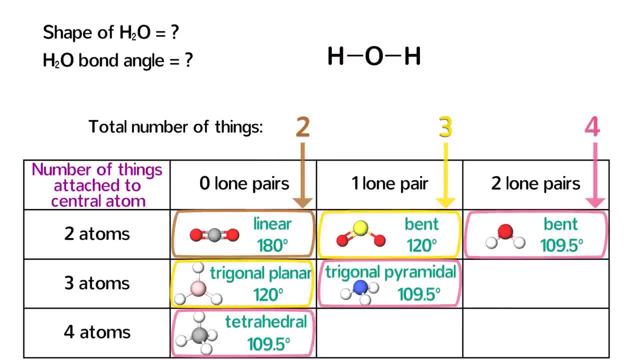 Oxygen is in the middle and there are two single bonds to the hydrogens. This leaves four valence electrons which we put as lone pairs on oxygen, giving it an octet. The structure has two bonded atoms and two lone pairs attached to the central. 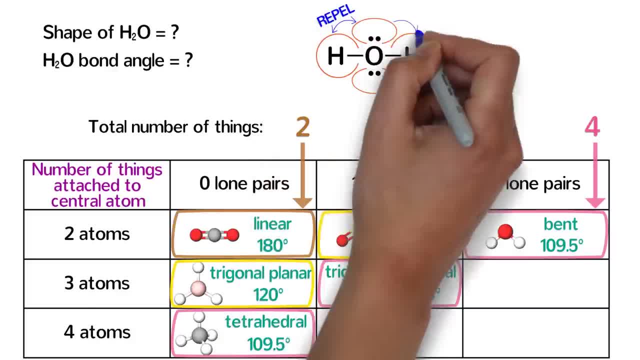 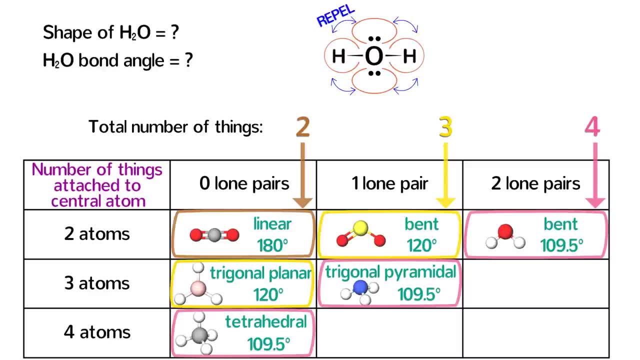 atom, for a total of four things that all repel each other. Just like in methane, these things will move as far apart as possible in three-dimensional space. The hydrogens can move away from you and the lone pairs can move toward you.